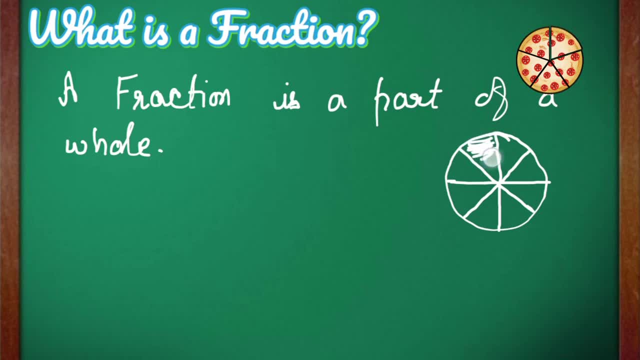 So this pizza have been divided into 8 equal parts, And if we eat one piece, how many parts remain? 7 equal parts will remain. So here, to express the eaten part in the form of fraction, we will write it as 1 by 8.. Or we can say we have eaten 1 out of 8 pizza slices. 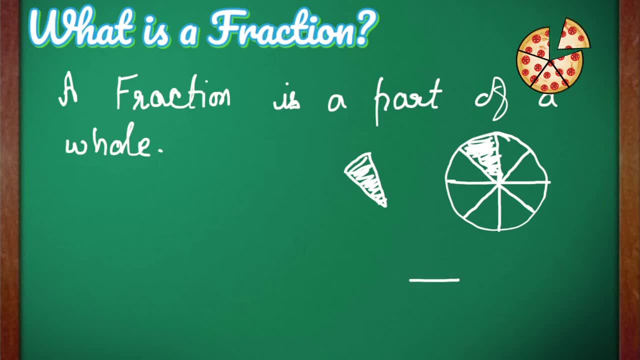 So for this we will write, We will write the total number of parts in the denominator. So here, the number written under the line is the total number of pieces, which is called as denominator, And the number written above the line is called as numerator, which is the piece of the pizza that we have eaten. So it is written as 1 by 8.. 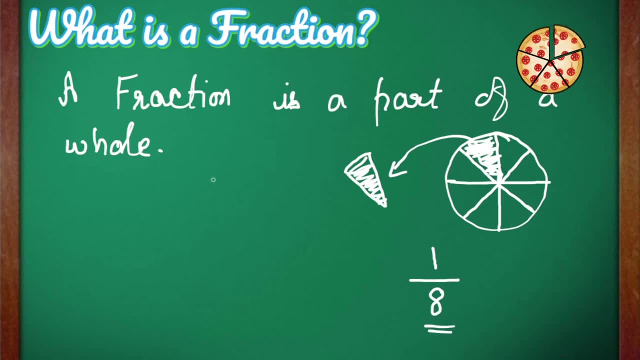 Or it can also be read as 1 out of 8 pieces. Now for second example. let us take apple. If this apple is divided into 2 equal parts and one part have been used have been eaten, Then half of the apple is eaten and half of the apple is remaining. 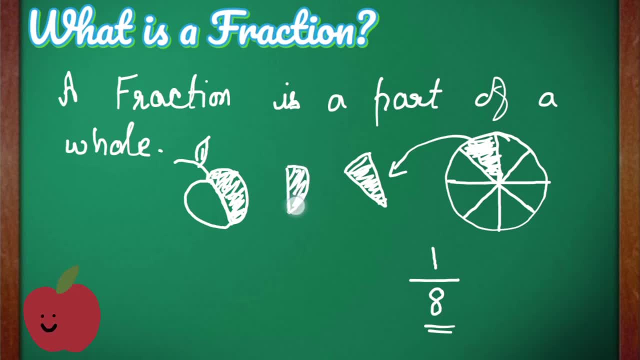 Now to express the eaten part in the form of fraction, we will write: To write this eaten part of the apple in the form of numbers, we will write it as 1 out of 2 pieces. So here again, below the line that is in the denominator, we will write the total number of pieces. 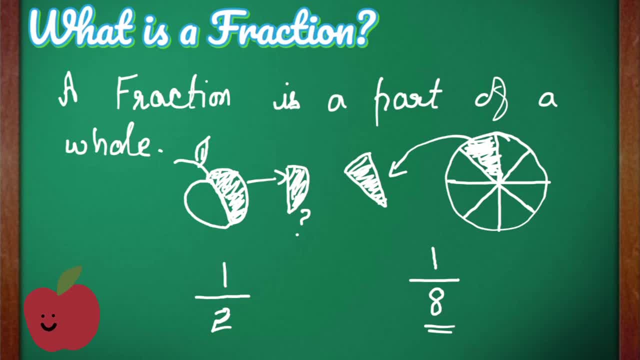 Total number of equal pieces, that is 2.. And in the numerator we will write the number of pieces that have been used, that is 1.. So this has been written as 1 by 2 in fractions. So this is how we can write the fractions.